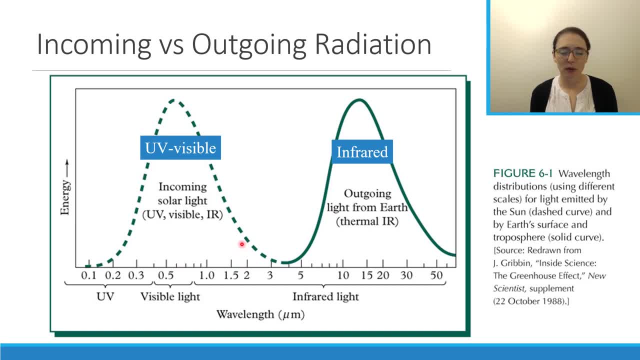 in the UV invisible wavelength. There's a little bit of contribution from the near IR, but it's primarily centered around the visible wavelengths of light. Now the Earth and the atmosphere absorb this solar radiation and then it's re-emitted as thermal infrared radiation. So the outgrowing 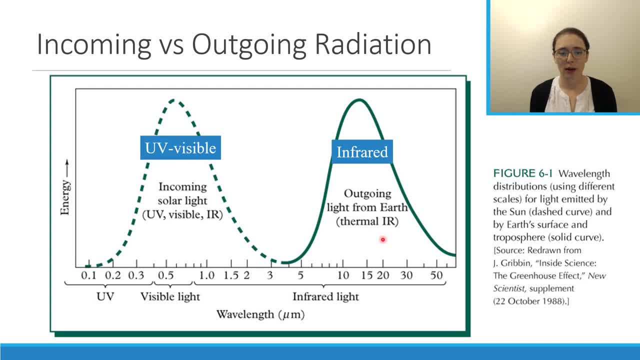 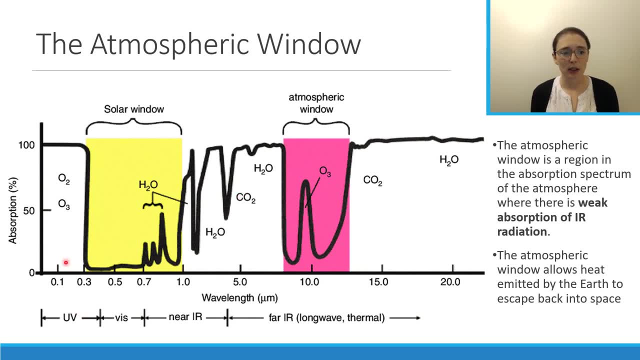 terrestrial radiation from the Earth is in the thermal infrared region. Now, there are a lot of species in the atmosphere that absorb radiation. In the UV region we have oxygen and ozone. Remember the ozone layer is absorbing UV light, preventing it from reaching the surface and giving us all 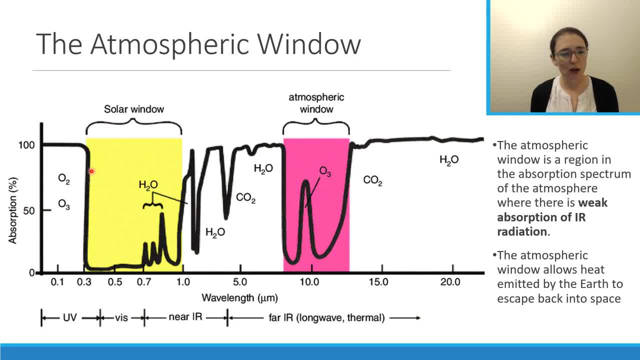 sunburns. And then we have the solar window, which is a region of relatively low absorption where solar light is able to really penetrate through the atmosphere. There's definitely wavelengths where there's almost zero percent absorption by the atmosphere, And then we have the atmospheric 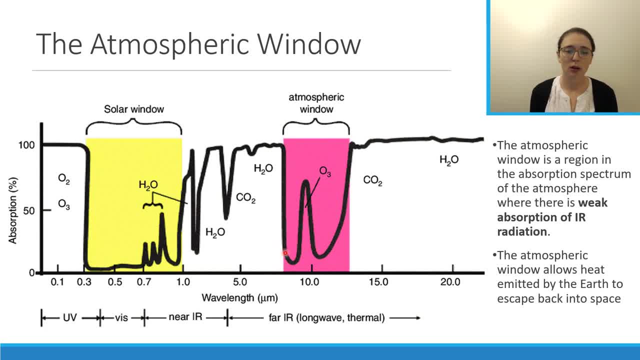 window, which is a region in the infrared region where there's also pretty good transparency to IR radiation. Now you'll notice one thing about this figure: There's lots of peaks from H2O, Lots of water peaks showing up here. The atmospheric window is essentially a window in the atmosphere. 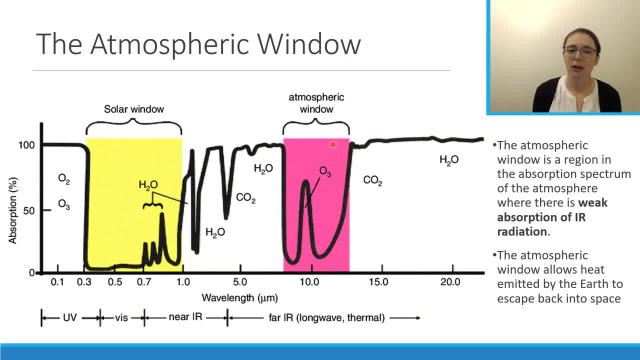 where there's water vapors, IR spectra, And the reason there are so many or the water peaks are so intense is because there's so much water in our atmosphere. The troposphere can be about three percent water by mass, So there's just lots and lots of water vapor in our atmosphere and that is. 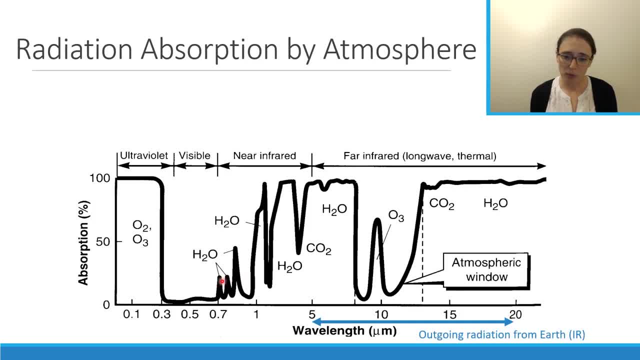 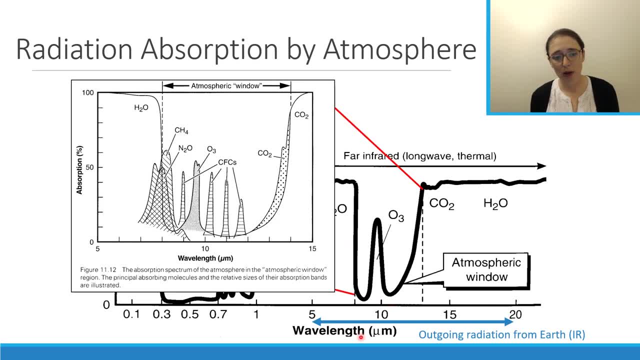 why it absorbs so strongly. Now within this atmospheric window. there are some species that do this, So you'll notice these are some of our greenhouse gases: Carbon dioxide, CFCs, ozone, nitrous oxide and methane absorb within the atmospheric windows. This is why these species 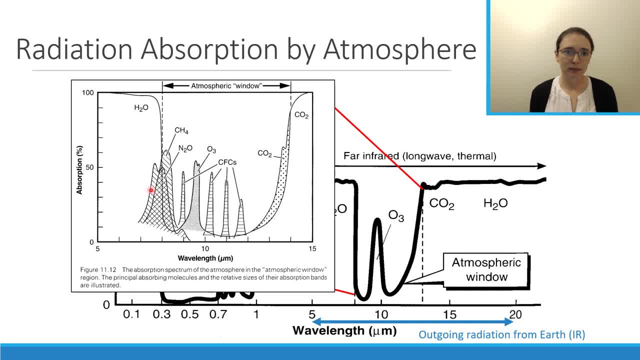 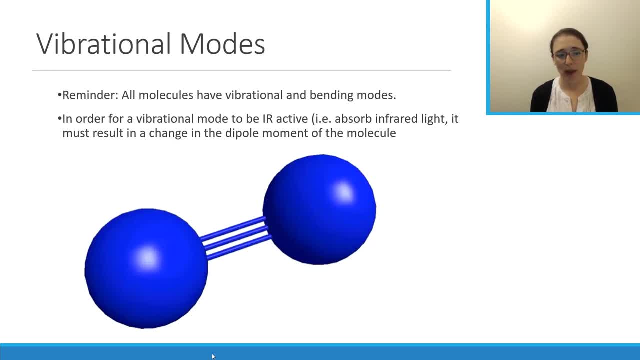 in particular, have such a big effect on climate. All right, so this is a chemistry class. Let's talk a little bit about why these species absorb infrared light. Why do some species absorb it? Why are others transparent to it? So, just as a reminder from probably genchem, but also PEBI, 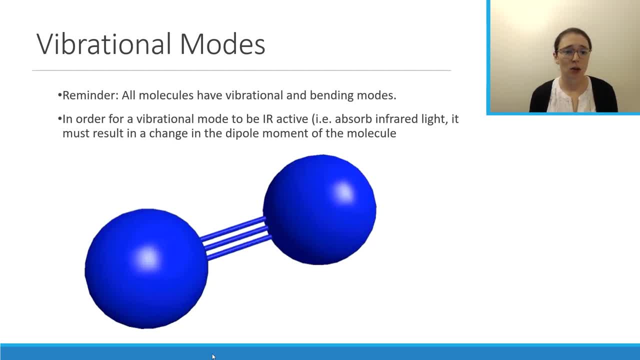 chem. all molecules have vibrational modes And in order for a vibrational mode to be IR active, that is, absorb infrared light, it must result in a change in the dipole moment of the molecule. So this is a video of the vibrational mode of nitrogen and two, and you'll notice, there's no. 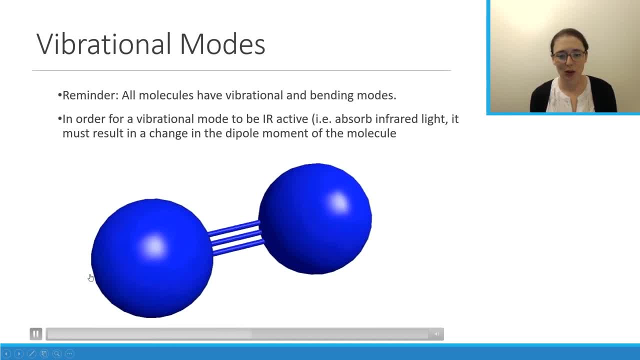 change in dipole moment, because there can't be. These are two nitrogens. There's no change in the polarity of the molecule here. So nitrogen is a very important molecule. Nitrogen is a very important molecule. Nitrogen is a very important molecule. Nitrogen and oxygen do not absorb in. 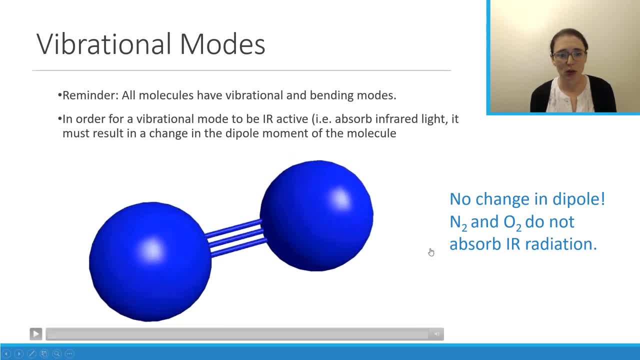 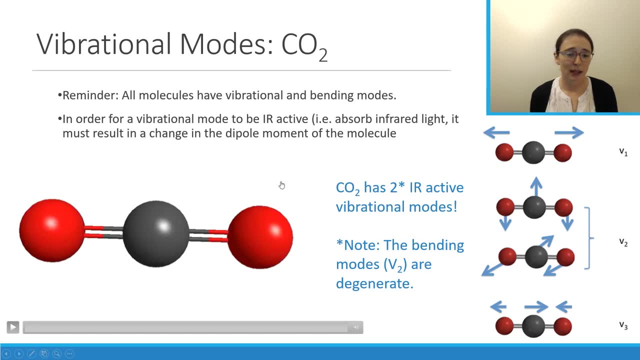 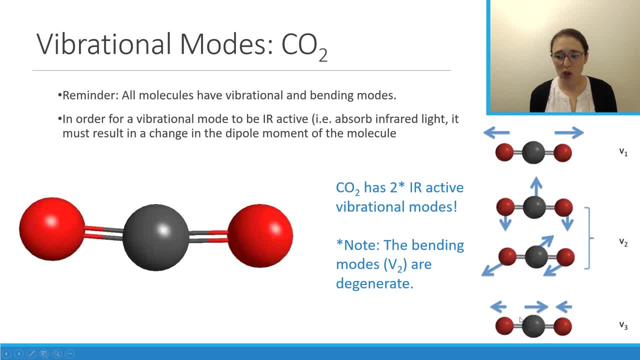 symmetric stretch, an asymmetric stretch and then two bending modes Play that one more time. So the asymmetric stretch and the bending modes are IR active because they result in a change in the dipole moment of the molecule. The symmetric stretch, however, does not. Now these two bending 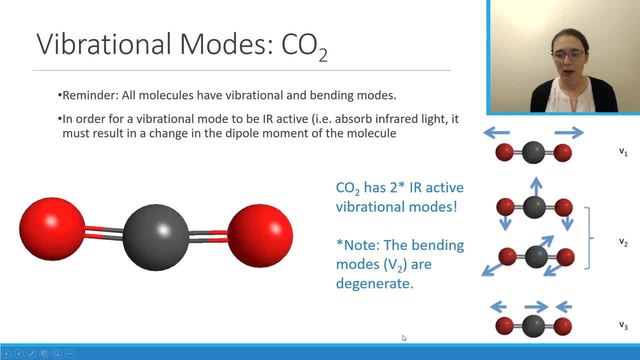 modes are degenerate, So they kind of only count as one mode. they absorb with the same wavelength, Because one of them is bending in the z direction and the other is bending in the y direction. So they're like the same mode basically it's just two different directions. So this is why carbon. 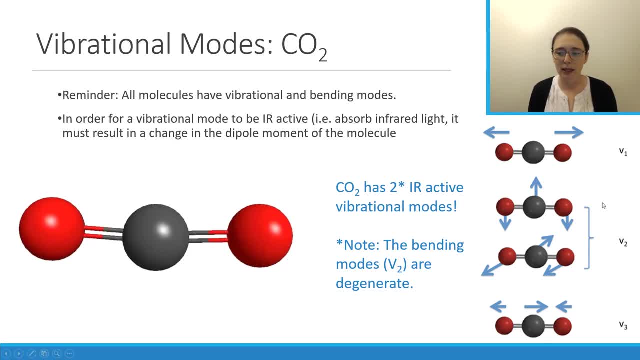 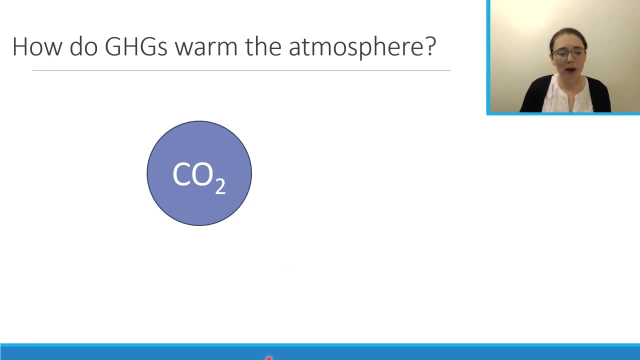 dioxide absorbs infrared light, and these absorptions of these two absorbing modes happen to be in the atmospheric window. So how do you know that these are the different modes or that they, greenhouse gases, actually warm the atmosphere? well, so we have our thermal radiation being emitted from the earth, that's our ir light, and it gets absorbed by this greenhouse gas molecule. 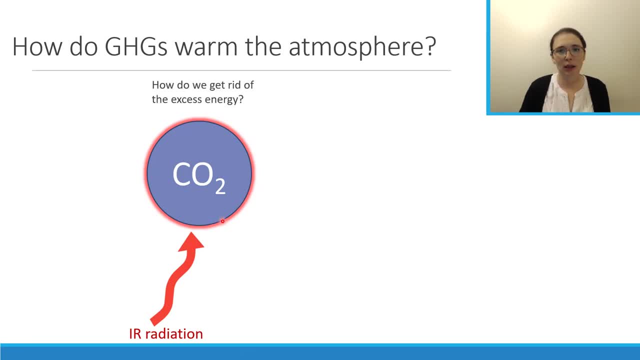 in this case carbon dioxide. now the co2 needs to get rid of this excess energy, so it's going to be re-emitted. but it can be re-emitted in any direction. so if it gets re-emitted upwards, it continues its path, trying to escape out of the atmosphere. but if it's re-emitted downwards it can. 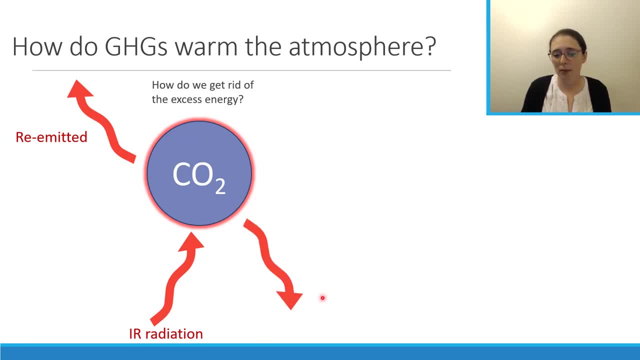 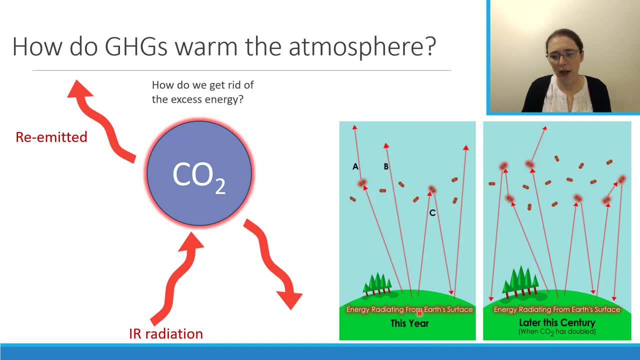 actually be either reabsorbed by the earth's surface or absorbed by other greenhouse gases that are in the atmosphere. so this is kind of what this looks like, where we have our infrared light being emitted from the earth's surface. it can get absorbed and then remitted upwards. 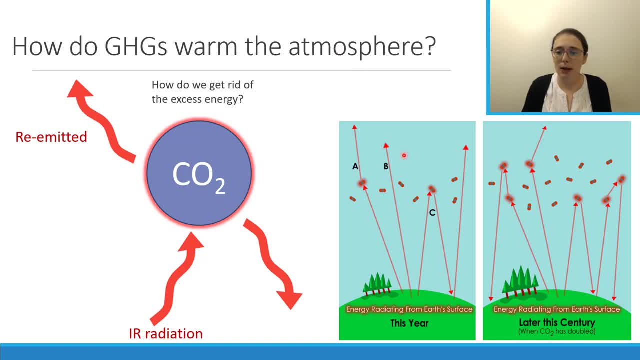 where it escapes. it can just make it through. it might never encounter a molecule of co2, or it can be absorbed and emitted downwards back to the earth's surface. now, if we add more co2 to the atmosphere, we see the probability of it being re-emitted downwards, or being even re-emitted and then reabsorbed by another molecule, is much higher. 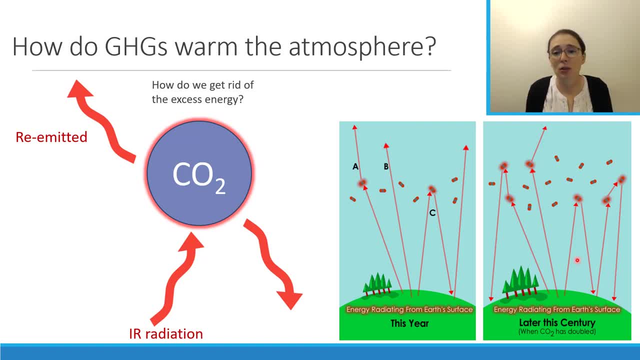 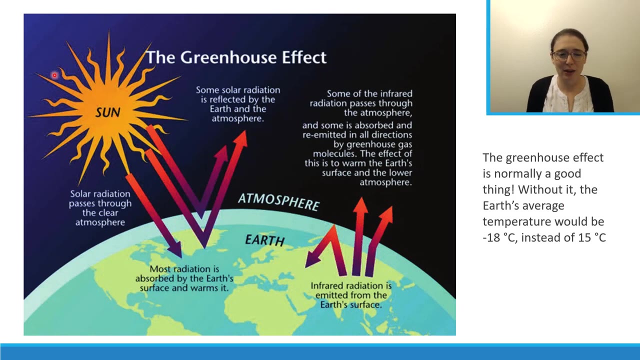 the more co2 we have in the atmosphere. beer's law applies to the atmosphere. actually, the absorption is going to be proportional to the concentration of the species in the air. all right, so now we get to the greenhouse effect. so this is our classic greenhouse effect diagram. solar radiation passes through the earth. some of it is reflected by the atmosphere. 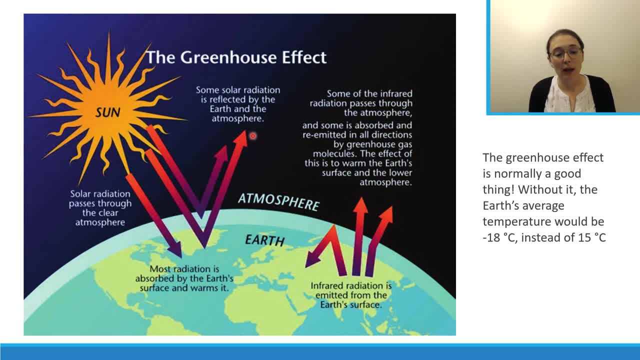 some of it's reflected by the earth's surface. light colored surfaces like sea ice and snow will reflect light. we also have clouds and aerosols that reflect some of the solar radiation, but a lot of it actually gets absorbed by the earth's surface and warms it. then that infrared radiation, that thermal heat, gets emitted from the earth's surface. 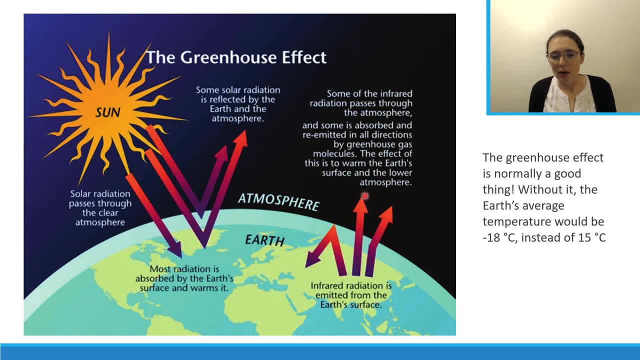 some of it's able to make it straight through the atmosphere back out into space. some of it gets absorbed and re-emitted back to the surface, and some of it gets absorbed, re-emitted but still is able to make it out. now, the greenhouse effect is a good thing. without it, the earth's average temperature would actually be negative 18 degrees. 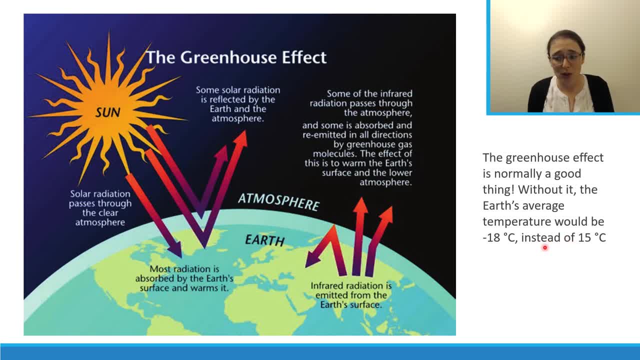 celsius, so very, very cold. our actual temperatures, average temperature is about 15 degrees celsius. that's much, much warmer. later on in the quarter we'll actually do some of the math and derive these numbers. but basically the greenhouse effect makes the earth habitable and actually our biggest. 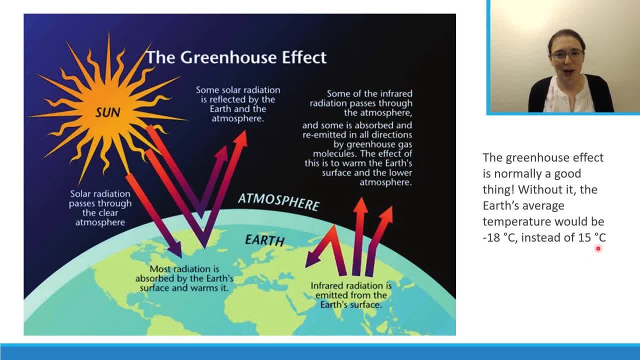 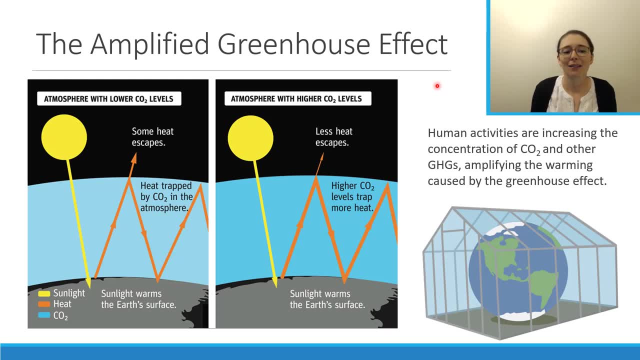 greenhouse gas is actually water vapor. um, water vapor traps a lot of the earth's radiation. now the problem is that anthropogenic activities are amplifying the greenhouse effect, so normally we have some heat escaping. co2 traps, some of the heat, but also a fair amount of it. 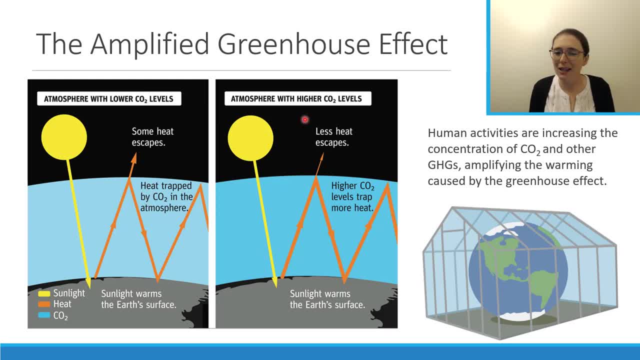 escapes. so normally we have some heat escaping. co2 traps, some of the heat, but also a fair amount of it escapes. now I just want to highlight that some of these temperatures are beingheated. as we increase co2 levels in the atmosphere, less heat is able to escape out into space. 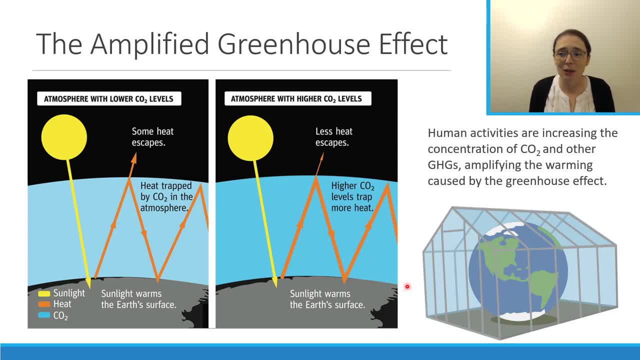 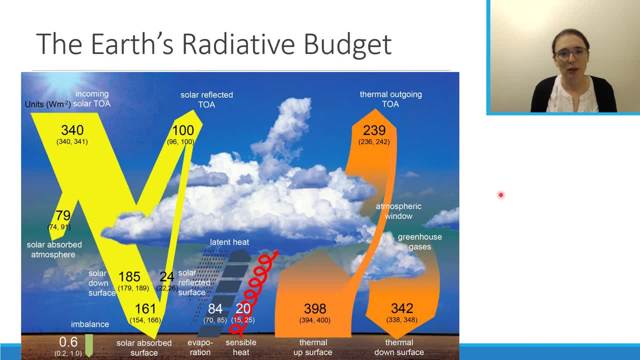 and this is going to cause warming of the earth's surface, the oceans and the atmosphere. so this is a diagram showing the earth's radiative budget. so this is essentially the transport of energy through the atmosphere, through all these different processes. so this looks really complicated, but i'm going to walk you through it. so we're starting with incoming solar radiation. 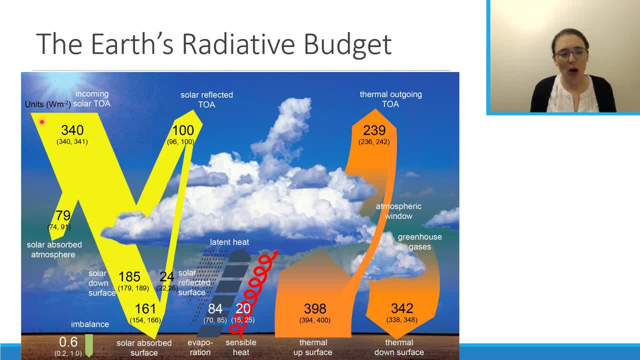 and all of these units are going to be in watts per meter squared. so on average we have 340 watts per meter squared of incoming solar radiation at the top of the atmosphere. that's what toa stands for now. the atmosphere absorbs about 80 watts per meter squared. 79 watts per meter squared. 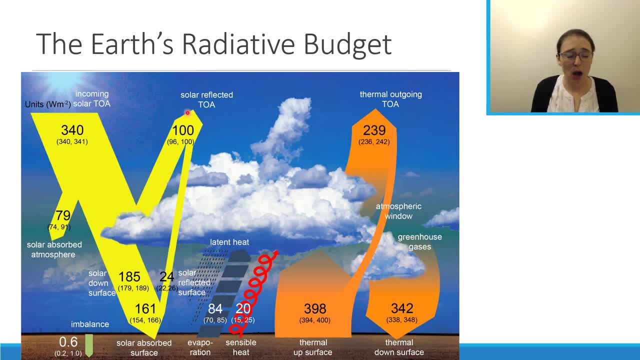 of that radiation- about 100 watts per meter squared- is actually reflected by clouds and aerosols and also the earth's surface, and that leaves about 160 or so watts per meter squared that are actually absorbed by the surface. now the earth needs to get rid of some of this energy. some of it goes into evaporation and 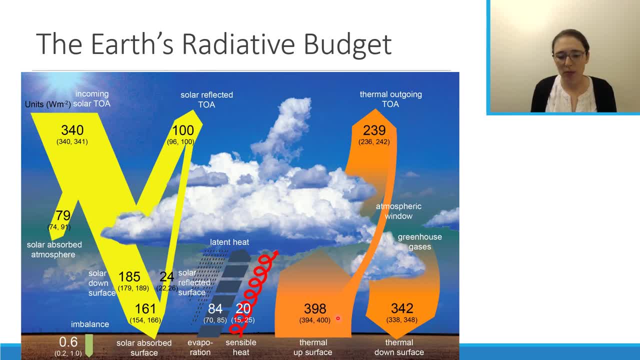 sensible heat, but most of it is going to be emitted from the earth's surface. now, if you look at this number- 161 in 398 out- that's really high. what's going on? well, a lot of the energy that gets reabsorbed from the atmosphere is going to be in the atmosphere through the greenhouse gases. 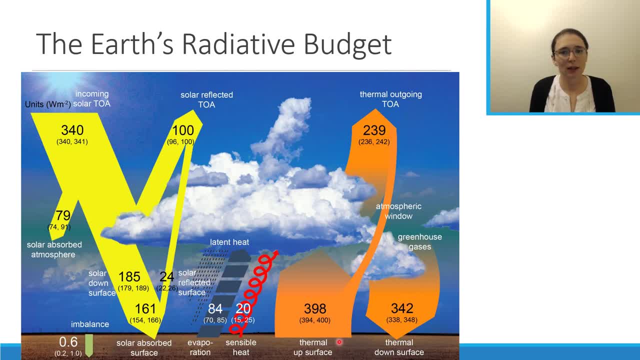 and reemitted, gets reabsorbed and then it has to come out. so this cycle- here the 398 to 342 arrow- is actually showing basically the cycling of energy that is trapped in the atmosphere by their greenhouse gases. now some of this energy actually makes it out through the atmospheric. 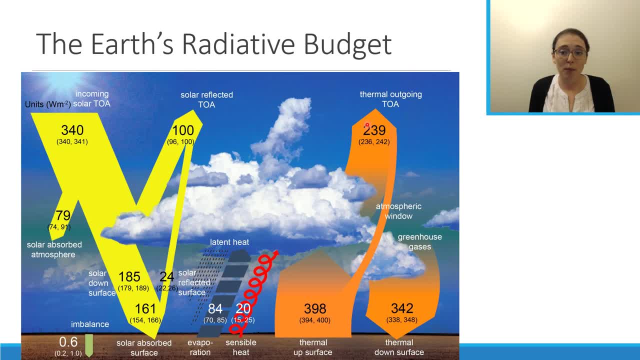 window, it's able to get basically straight out of the atmosphere and then some of it gets basically reemitted upwards, resulting in 239 watts per meter squared of outgoing thermal radiation at the top of the atmosphere, of the atmosphere. Now, in order for the Earth's energy balance to be our energy, 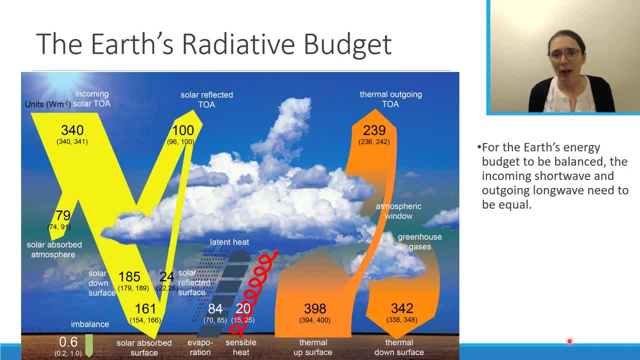 budget to be balanced, the incoming shortwave and outgoing longwave need to be equal, So we need to have the downwelling shortwave equal to our upwelling longwave, Or in other words, energy in needs to equal energy out. So 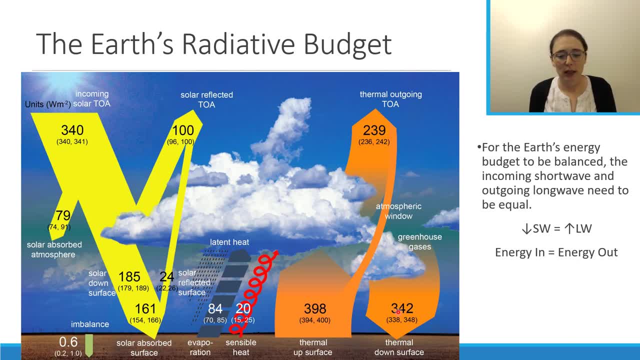 these measurements of the absorption and re-emission by the Earth's surface are actually. we're actually pretty uncertain about some of these numbers. But what we aren't really certain about is these top of atmosphere numbers, because we measure these from satellite And we have lots of satellites orbiting the Earth. 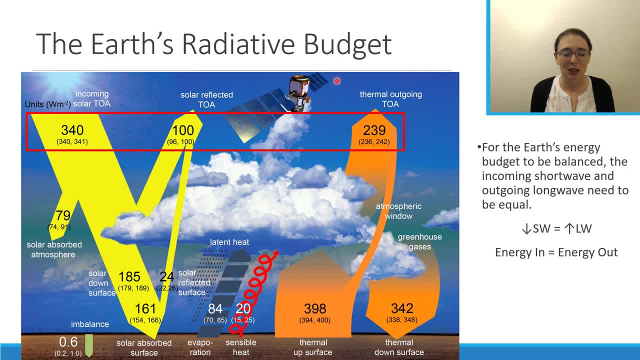 actually taking these measurements and they've been doing it since 1980. So we have a pretty long record going back. So we're actually pretty confident about the incoming solar. So we're actually pretty confident about the incoming solar. So we're actually pretty confident about the incoming solar. 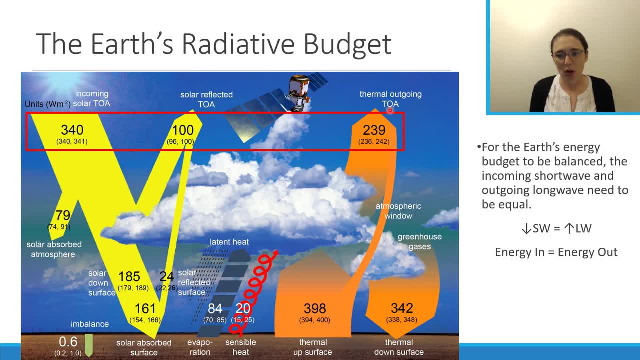 The amount that gets reflected in our outgoing thermal radiation. Now, if we sum all these things up, we'll see 340 incoming and then a hundred of that is just reflected. it doesn't get absorbed. So in that case we have 240, that is. 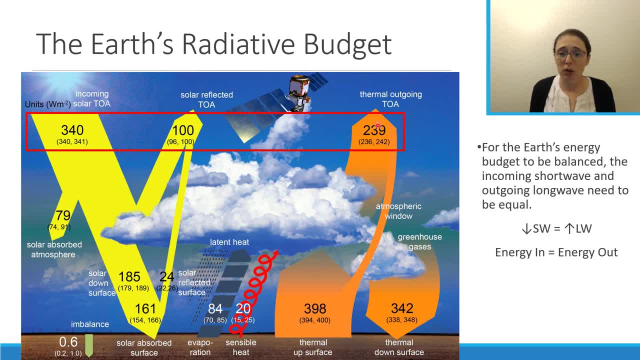 going to get absorbed: 240 watts per meter squared. Now the thermal outgoing radiation is 239 watts per meter squared. So we're actually pretty close to energy in equals energy out. Now it's a little tricky calculating the exact energy imbalance, because it's pretty small and these numbers aren't that sensitive. but 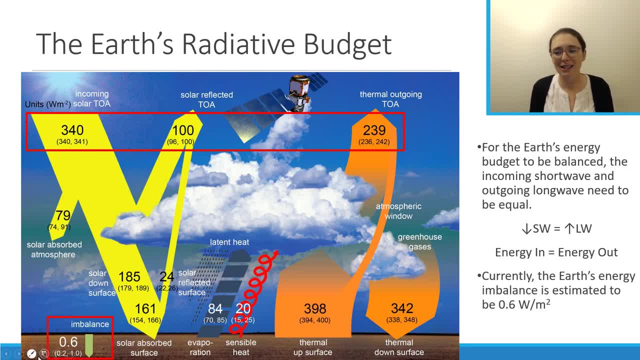 the best estimate is that we have an imbalance right now of 0.6 watts per meters squared, So essentially we're have about 340 coming- or sorry, 240- coming in and getting absorbed, but only about 239 going out. And the best estimate 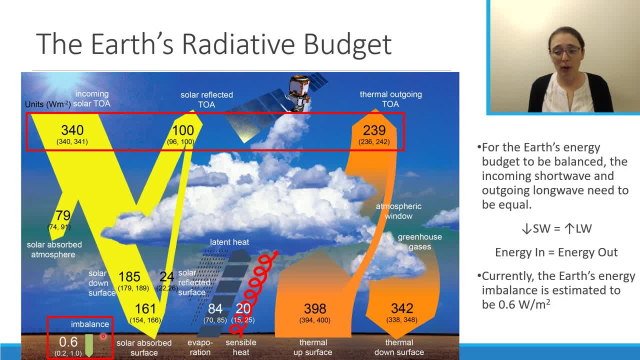 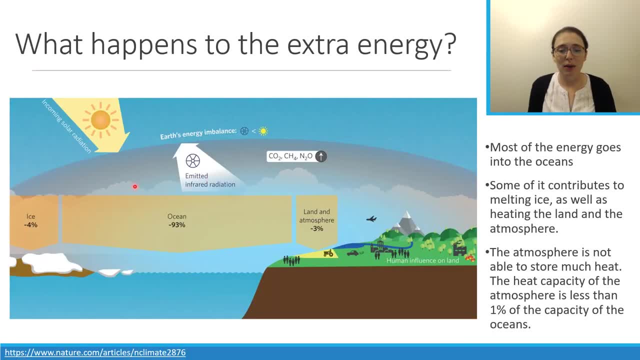 for that exact number is 0.6 watts per meter squared of energy imbalance. so then, where is this extra energy going? well, 93% of it gets absorbed by the oceans and it goes into heating the oceans. about 3% heats the land in the 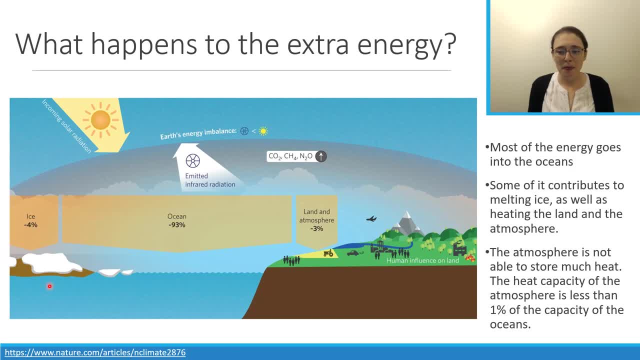 atmosphere and about 4% goes to melting ice. so we think about the heat capacity of water. versus air. water has a much higher heat capacity and actually the heat capacity of the atmosphere is less than 1% of the total of the oceans. so that's why so much of this energy is actually ending up in the oceans. the 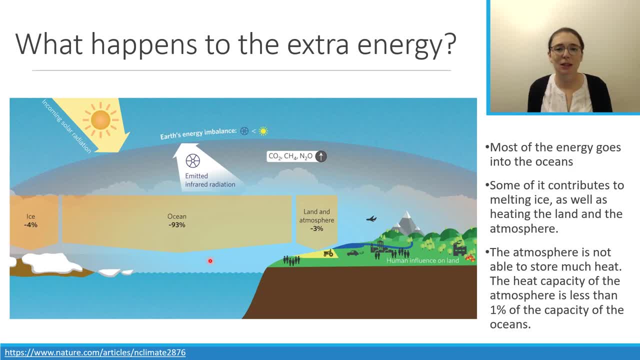 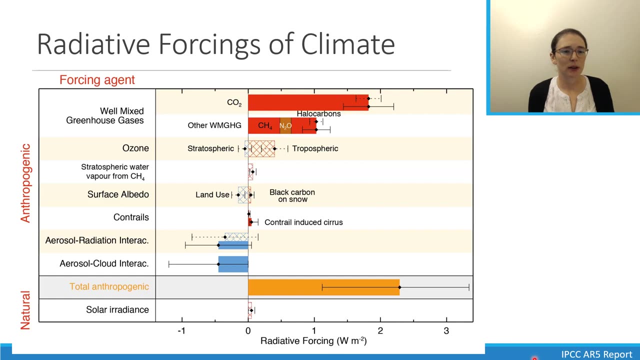 ocean temperature has only risen a little bit, but because the specific heat of water is so high, it actually. this actually converts to lots and lots of radiation- sorry, of energy- being absorbed by the oceans. all right, so switching gears here a little bit, now we're going to talk. 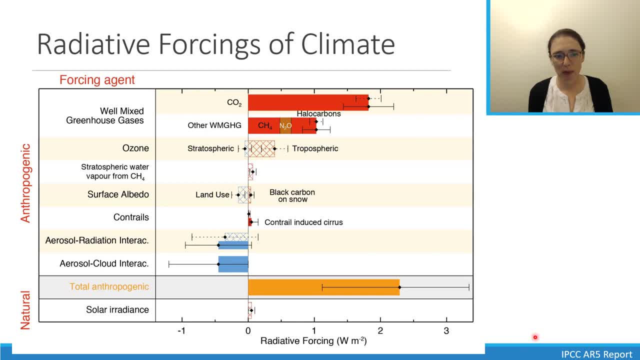 about the heat of the atmosphere and we're going to talk a little bit about radiative forcing. so professor Prather has shown this plot before. basically, what we have here is our different forcing agents, so carbon dioxide, our other WMG, HD is well mixed greenhouse gases, so our other greenhouse gases: ozone. 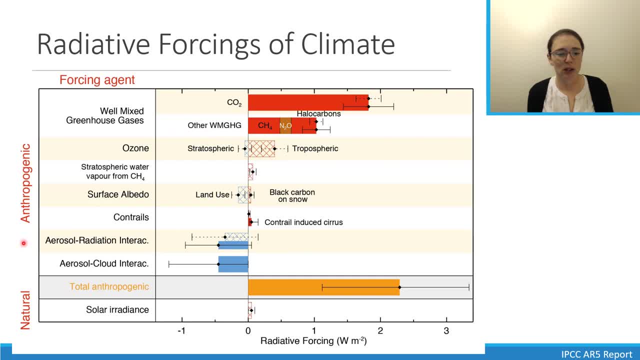 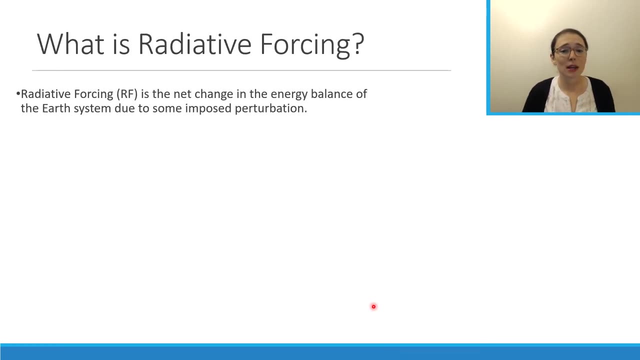 surface albedo aerosol radiation interactions and aerosol cloud interactions, and then each of these is showing shown as the radiative forcing in watts per meter squared. so you might be wondering what exactly is radiative forcing? it's basically the net change in the energy balance of the earth system due to some perturbation. it's expressed: 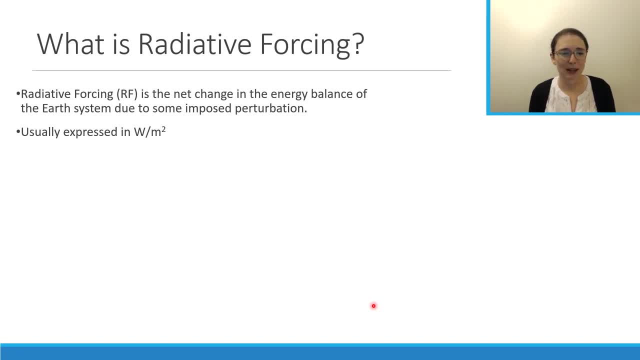 in watts per meter squared almost always. sometimes you might see it in like milli watts per meter squared, but those are the standard units. enforcings are presented as usually as a value due to changes between two times. so the most common is going to be pre-industrial to present-day. 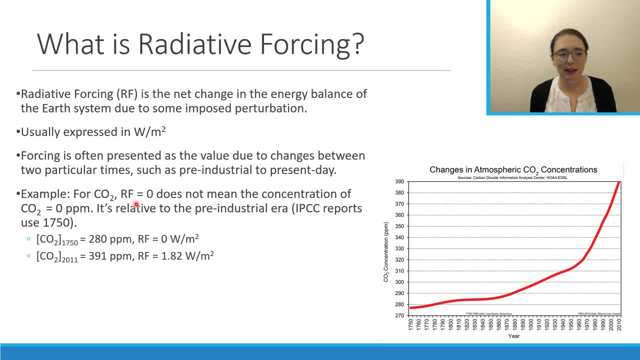 so what this means is that for carbon dioxide, a radiative forcing of zero does not mean that the concentration of co2 is zero parts per million. it's relative to the pre-industrial era, which the IPCC reports define as 1750. so in 1750 the 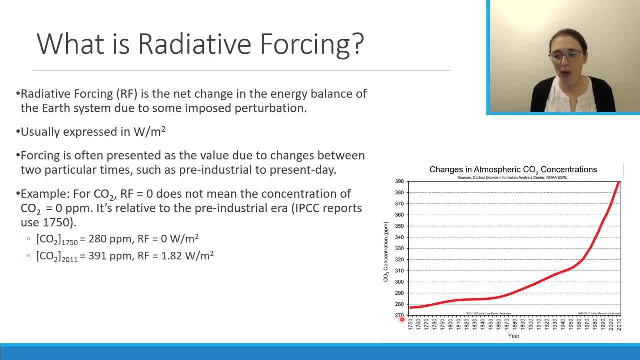 concentration of co2 was 280 parts per million. this is a plot of co2 over time. so we see 1750, we're at about 280, you know, within an error on this measurement. so the radiative forcing here is zero because this is what we've defined as our baseline. now, in 2011, the concentration of 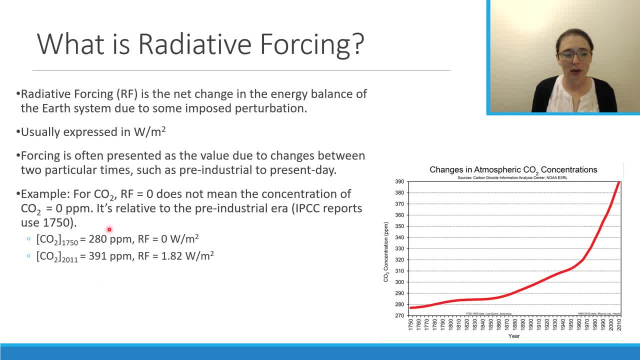 co2 is 391 parts per million, so much higher than the 280. so for that value a radiative forcing of 1.82 watts per meter squared was calculated. now, a positive radiative forcing indicates a warming perturbation. a negative radiative forcing indicates a negative radiative forcing indicates a negative radiative. 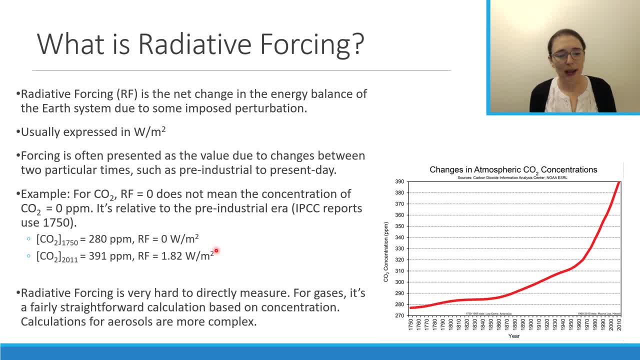 cooling perturbation. these numbers actually aren't directly measured. they're usually done as a calculation for gases. it's actually pretty straightforward. this is the equation for co2. the radiative forcing is just equal to some constant times the natural log of the current co2 concentration over the. 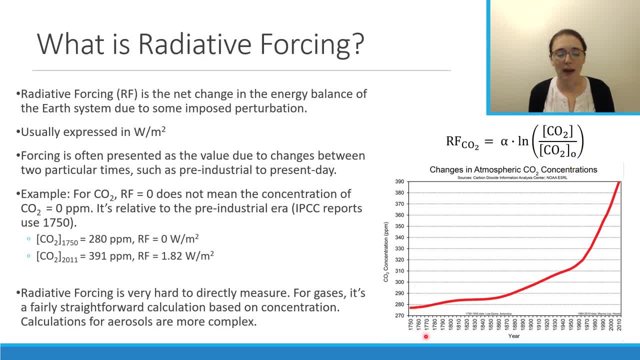 initial concentration, which would be our 1750 value. so to get this 1.82 number, all you would do is put in 391 over 280, take the natural log and then multiply it by whatever value of alpha you're using, I think the most commonly accepted value. 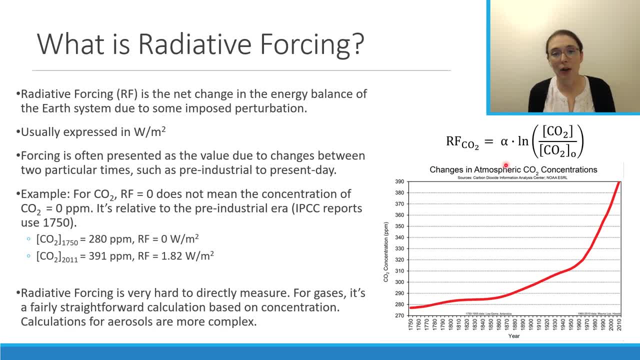 is like 5.35 or something, um. but this is like an active area of research actually, that people try to figure out the best parameterizations for these radiative forcing equations. now for things like aerosol and surface albedo, um, the calculations are a bit more complex and not straightforward, so we're just going to 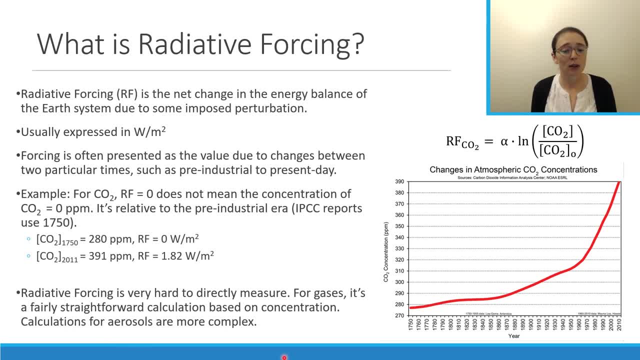 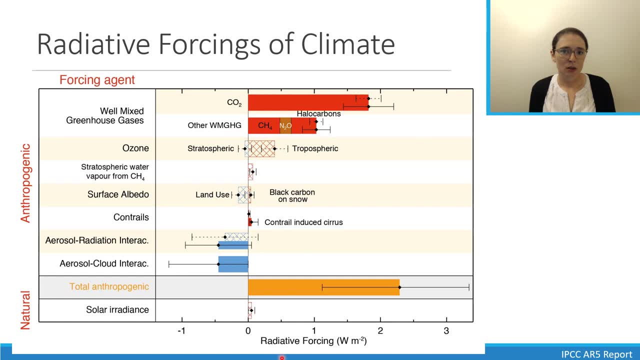 move forward. um, but the whole purpose of doing these is so that you can basically get one number that you can compare between all of these different perturbations to the climate system. all right, so back to our plot. we can see that carbon dioxide is the largest. 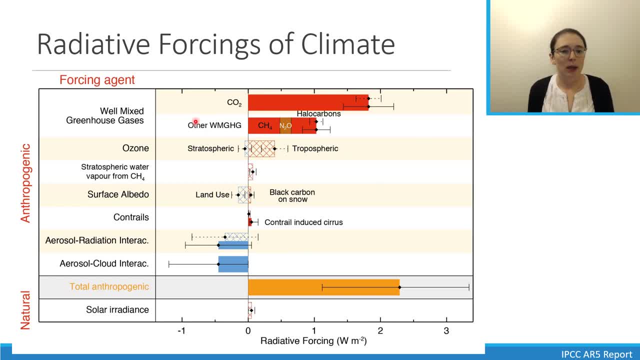 contributor to our radiative forcing. and then we have our other well-mixed greenhouse gases: methane, nitrous oxide, um, halocarbons, ozone is a contributor- tropospheric ozone- and then we have cooling effects. so negative radiative forcings from our aerosol radiation interactions in our 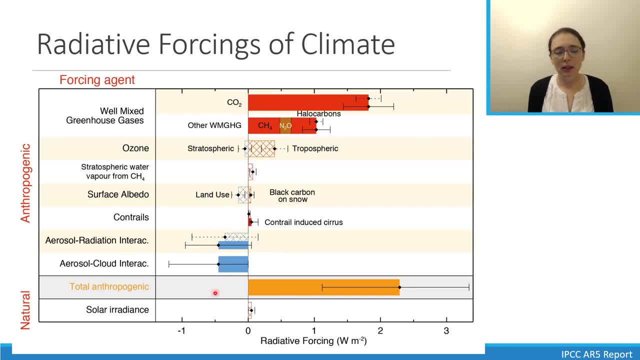 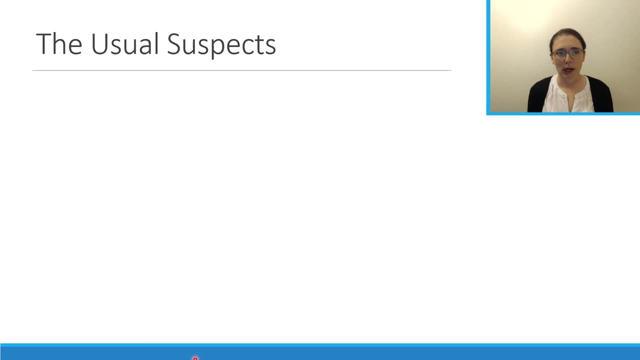 aerosol cloud interactions, and this leads to a total anthropogenic radiative forcing. um. it's positive, and it's about 2.4 watts per meter squared notice. there are pretty big air bars on this though. all right, let's talk about our major greenhouse gases, so obviously we 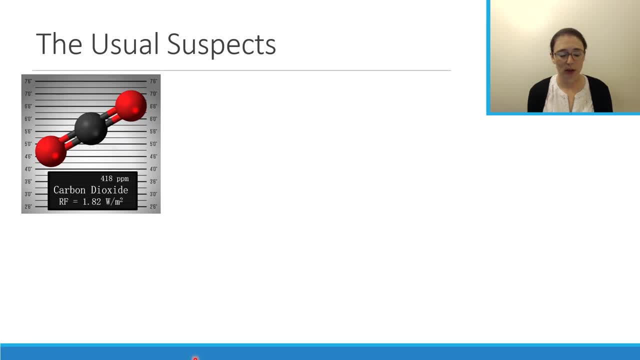 have carbon dioxide um. its current concentration is four point or sorry- parts per million, so that's significantly higher than our pre-industrial value of about 280 ppm, and its radiative forcing is estimated at 1.82 watts per meter squared. that's actually an old. 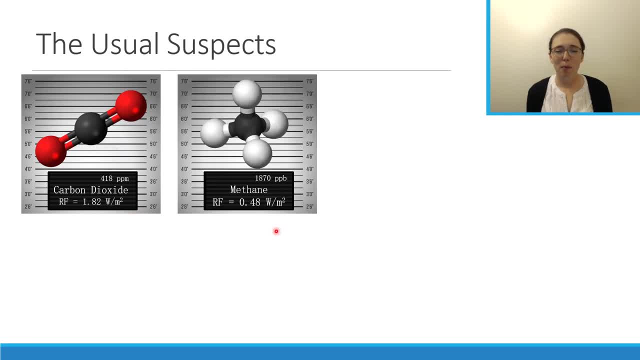 value. it's a little bit higher now. then we have methane, so the current concentration of methane is about 1870 parts per billion, 1.87 ppm, and it's rated forcing is 0.48 watts per meter squared. then we have nitrous oxide, with a radiative forcing of .17 watts per meter squared. so these 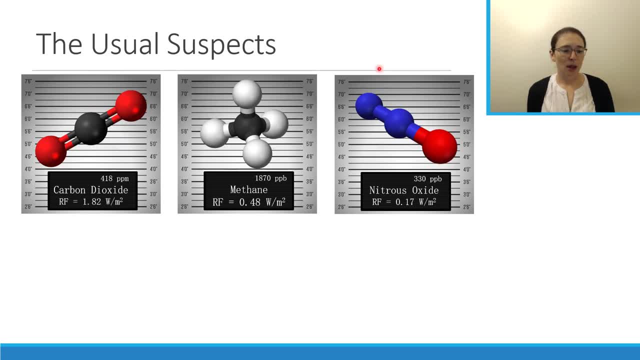 are on three of our biggest greenhouse gases. then we have our halo carbons, our halogenated compounds, so we'll remember these from our lecture on stratospheric ozone depletion. these include our CFCs, our hfcs, our hcfcs. in total, we have about 3600 parts per trillion. 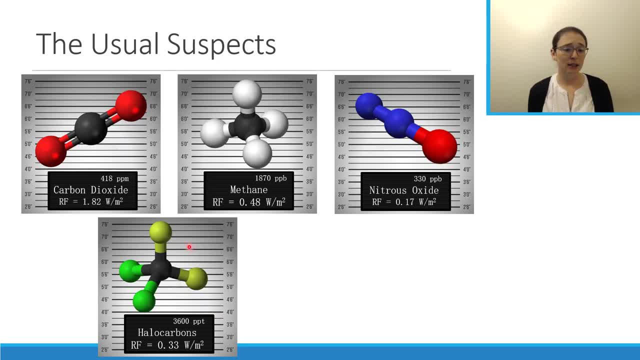 um of equivalents, but this is made up of dozens of compounds, so the individual concentration of these compounds is much lower, but in some this is the approximate concentration in total and their total radiative forcing is 0.33 watts per meter squared. so again, that's for dozens of compounds, not just a. 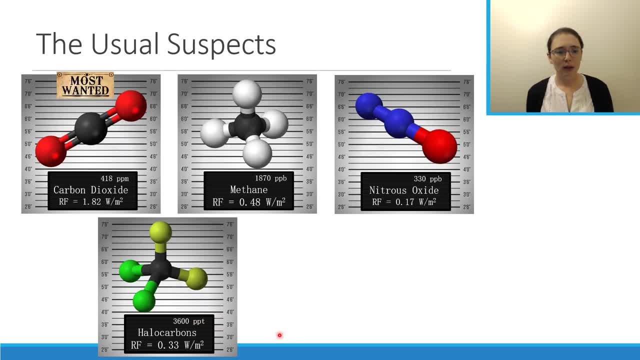 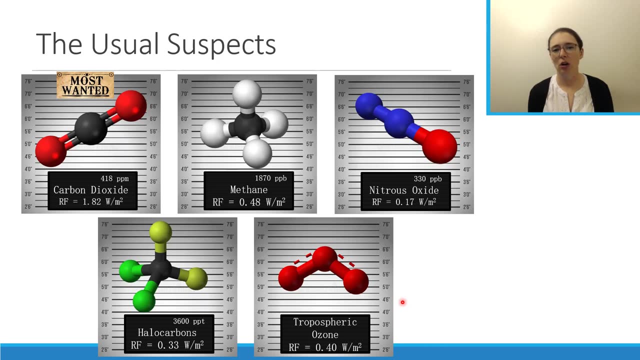 single compound. and then, finally, our last major greenhouse gas is going to be tropospheric ozone. so tropospheric ozone has a radiative forcing of about 0.4 watts per meter squared. now, we discussed the sources of tropospheric ozone in our lecture on air pollution. remember, tropospheric ozone is formed. 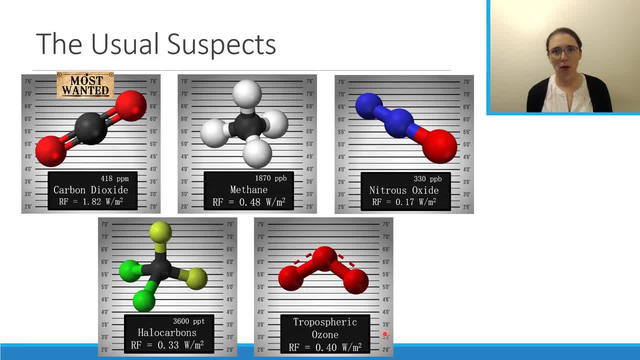 from photochemical smog formation from our ground level air pollutants which react in form ozone. so we've actually already covered the sources of two of these greenhouse gases. already I put a little most wanted sticker on carbon dioxide because obviously you can see here it is our largest single contributor to climate change and has the largest 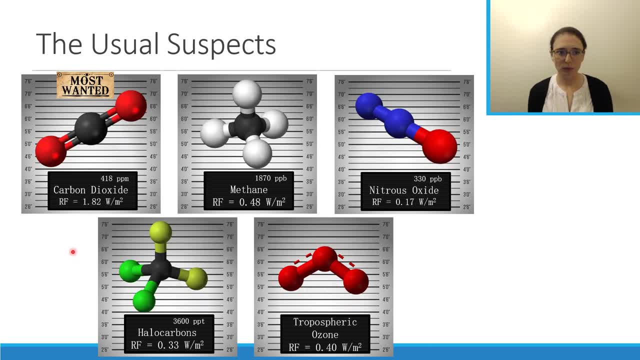 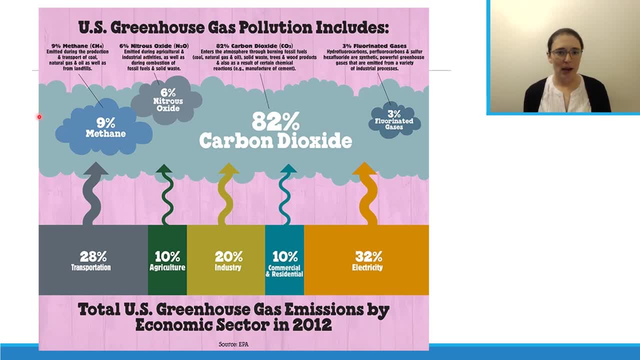 radiative forcing value out of all of these compounds. all right, let's talk about the sources of greenhouse gases. I like this graphic a lot. it's actually made by Ben and Jerry's. it's a little old- 2012- but it gets the point across. so. 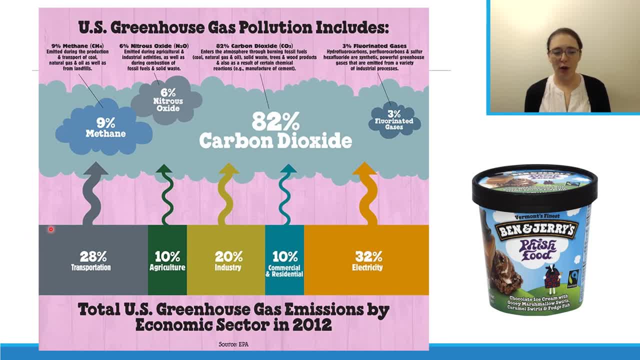 the sources of greenhouse gases in the United States. about a third are from transportation, so it's going to be our cars, buses, airplanes, trucks, etc. about 32 percent comes from electricity generation, so our power plants, and then the other third is split between agriculture, industry and commercial and residential. now the sources of methane are mainly from the. 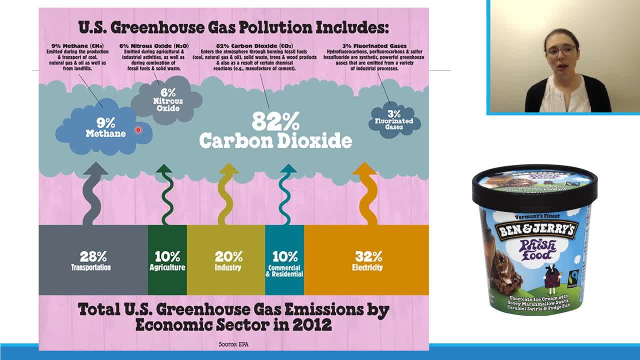 production of fossil fuels. so that's like extracting oil and natural gas results in methane leaks, as well as the mining and transportation of coal. we also get methane formed from anaerobic decomposition, so, for example, landfills, where things are organic matter is buried. there's not a lot of oxygen. 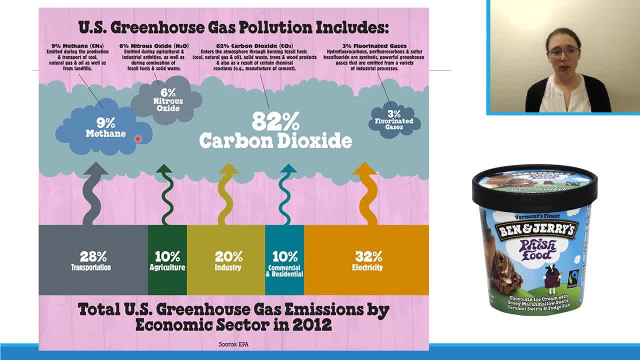 methane will actually be formed in landfills from waste disposal. then we have nitrous oxide and 2o. it's primarily actually emitted from agricultural activities and a little bit of a contribution from industrial activities and fossil fuel burning. carbon dioxide is our largest greenhouse gas, 82 percent. 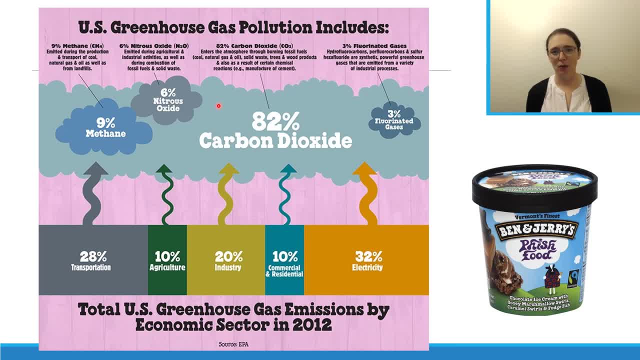 of total emissions, and it's primarily from the burning of fossil fuels. right, we're digging up solid carbon from under the ground and burning it and putting it into the atmosphere in absolutely massive amounts, so fossil fuel burning is by and far the largest source of carbon dioxide in our atmosphere. 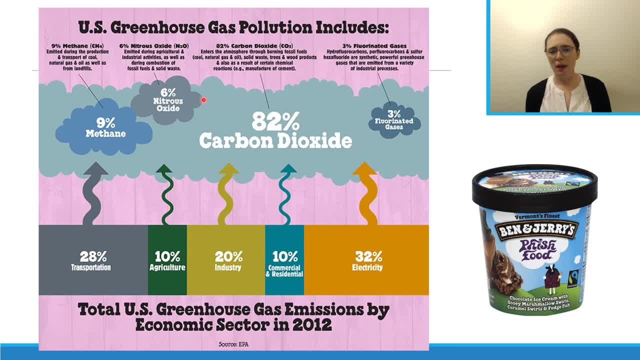 although there is also some contribution from, for example, waste disposal, from cutting down trees and wood, and also chemical reactions. and then our fluorinated gases. this is fluorinated- I would probably call this halogenated gases- but our CFCs, HFCs, sulfur, hexafluoride- are all synthetic compounds. 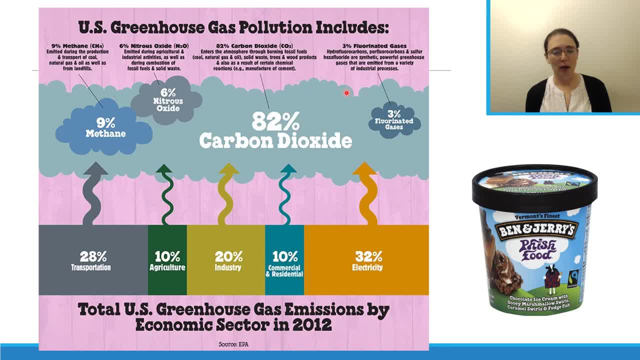 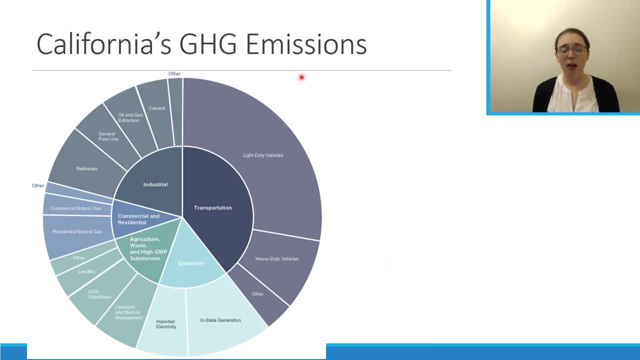 that are used for things like refrigerants, air conditioning and other processes. now this is a inventory of California's greenhouse gas emissions. we're pretty similar to the national average, the US average, but we have a bit more contribution- from transportation probably- than the rest of the country. 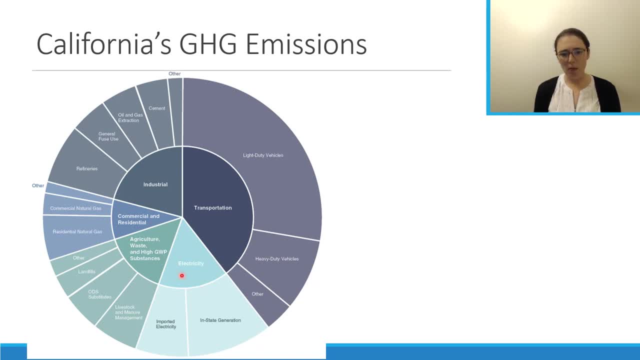 and maybe a little bit less than electricity. but one thing I wanted to point out is how big the contribution from light-duty vehicles is. in California, I mean, this is over 25 percent of our total emissions are actually coming from light-duty vehicles, which are normal cars. these aren't these. 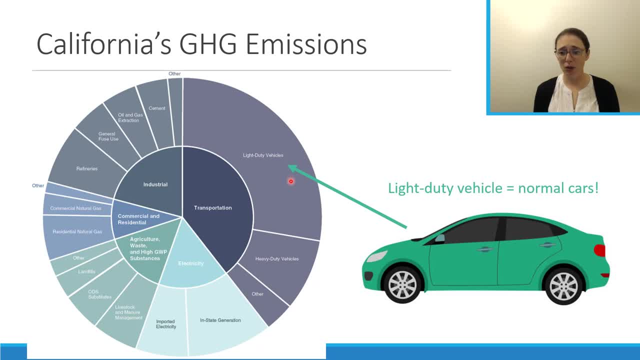 aren't trucks or buses or anything like duty vehicles, are passenger vehicles, so a really big contribution here of our total greenhouse gas emissions in California is coming from transportation. so next time you're feeling helpless, like you can't do anything about climate change, you know, ride your bike to the 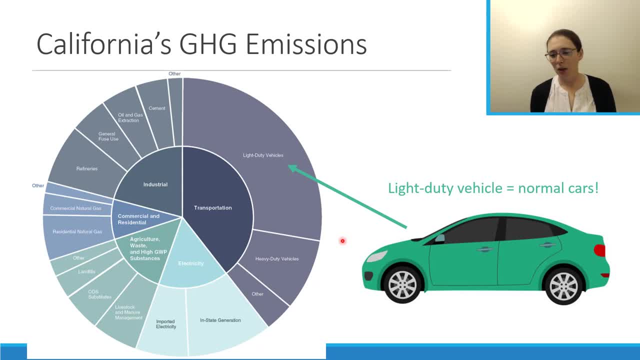 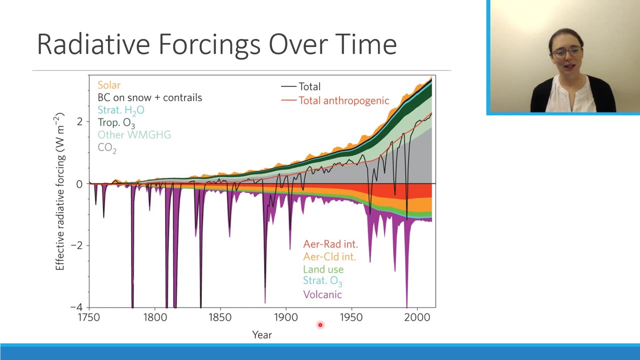 store. try taking public transit if you can afford it. maybe get a more fuel efficient vehicle that will really help cut down on our greenhouse gas emissions. okay, so switching gears. going back to radiative forcing, these are some estimates of the radiative forcing over time. I like this. 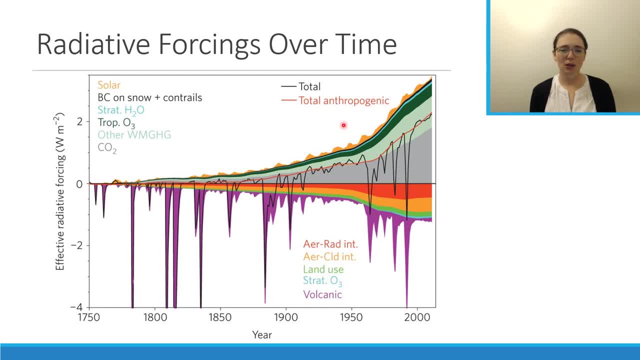 plot a lot because it shows the anthropogenic contribution as well as the total, which includes natural perturbations. so in gray we have carbon dioxide- this light green color is our other well mixed greenhouse gases. we have tropospheric ozone, black carbon, stratospheric water vapor which comes 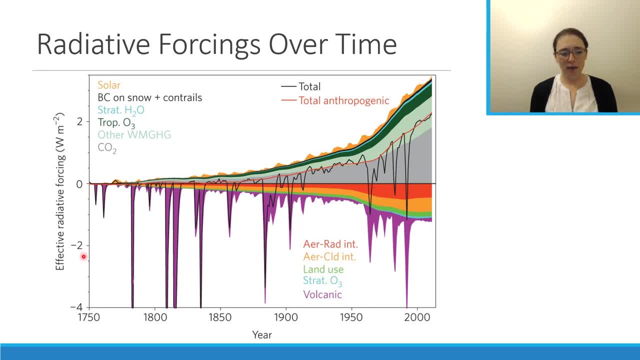 from methane. and then on our negative radiative forcing side, our cooling side, we have our aerosol radiation interactions, our aerosol cloud interactions, land-use changes, stratospheric ozone depletion and volcanic, and then up here for our natural we have in yellow solar. so I like this plot a lot because it shows the natural perturbations to the climate. 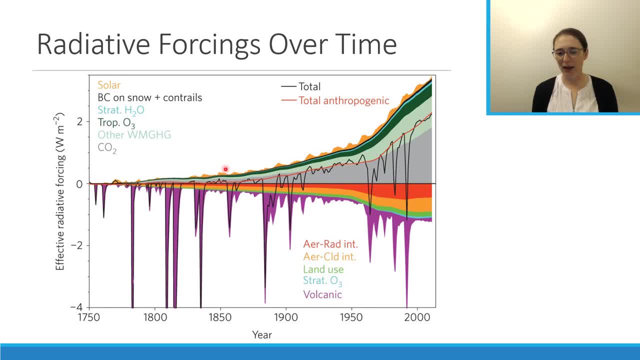 system happen, but they oscillate. right. the solar radiation doesn't really have a distinct upward trend. it goes up and then it goes down. it goes up and then it goes down. on this cycle the same with the contribution from volcanic right we have a big spike when there's a big volcanic eruption. we 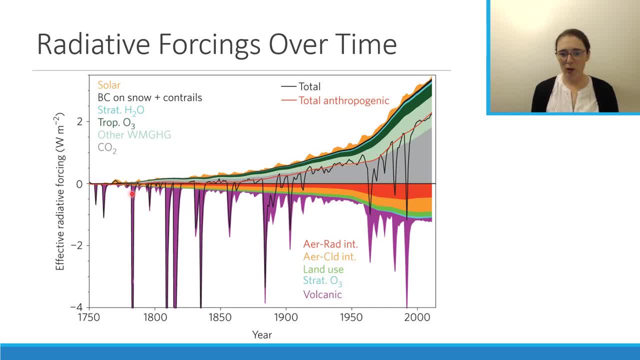 have a lot of sulfate aerosol emitted that reflects radiation, so we have a big spike and then it goes back to baseline- big spike, baseline, big spike, baseline, whereas with our anthropogenic greenhouse gases you can see that these are just accumulating in the atmosphere over time. the concentration is going up. 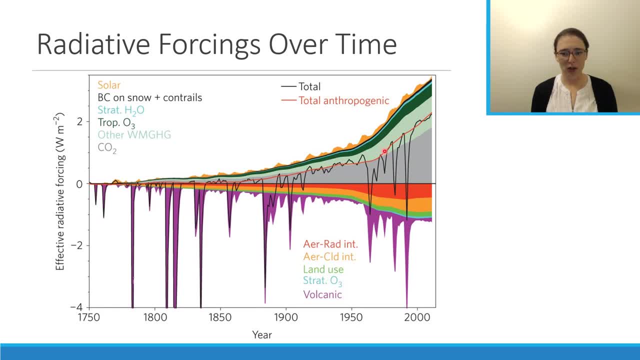 and up steadily and causing our total radiative forcing to go up and up. so this is really really compelling evidence that our changes in the climate system that we're seeing are really due to anthropogenic activities. the natural system is doing its thing. it's, it's oscillating and going back and forth, but it is not enough to overcome. 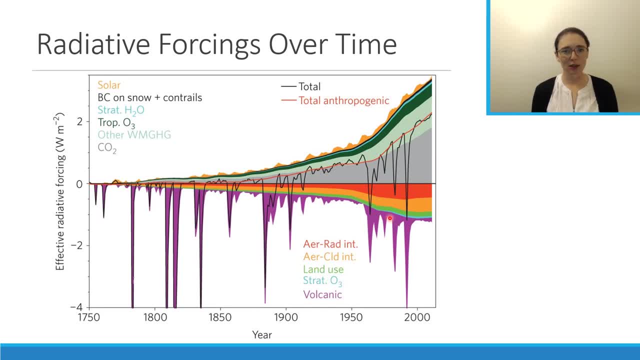 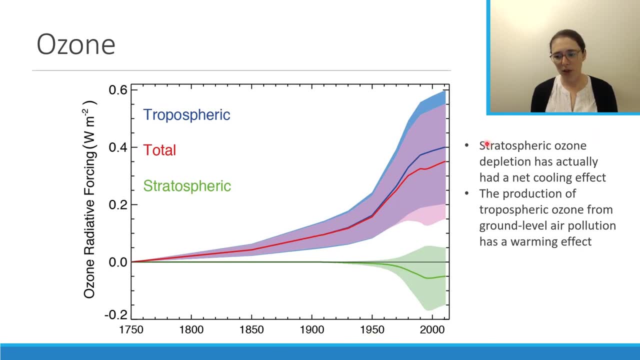 all of these anthropogenic perturbations to the system, all right. finally, the last thing I want to talk about is ozone. so stratospheric ozone depletion has actually had a net cooling effect. so we talked about ozone depletion. we talked about the ozone hole over Antarctica. there's also one that sometimes forms. 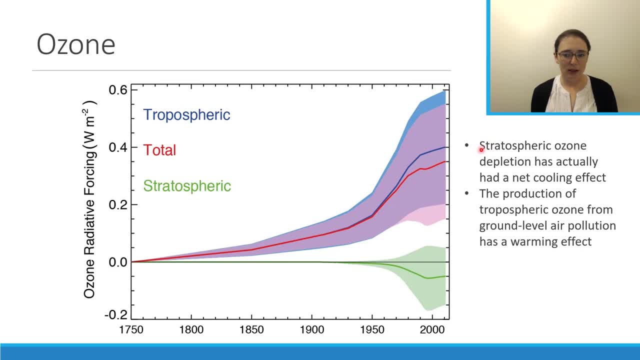 over the Arctic. that's not what's really driving this. I think there's been a depletion of about 4% on average over the whole stratospheric ozone layer due to chloroplurocarbons, so this depletion of ozone across the whole earth has actually had a net cooling effect. it's not very large, but it has had a net. cooling effect and while it's not getting worse- you know we have our Montreal Protocol kicking in in the late 80s and 90s- it is going to be slow to recover now. tropospheric ozone, which is produced from our ground-level air pollution, has a positive radiative forcing, so this has a warming effect. 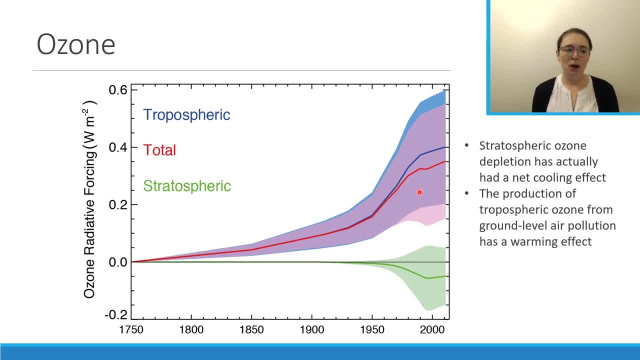 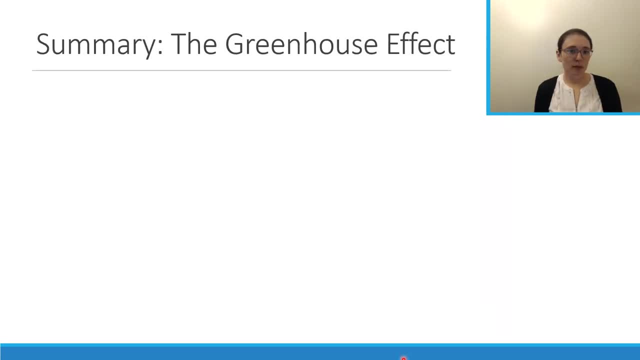 and it's much larger than the stratospheric ozone depletion. so overall ozone actually has a positive radiative forcing, which means it has a net warming effect. That is the end of lecture 6.2 on the greenhouse effect. I know this one was a long one. 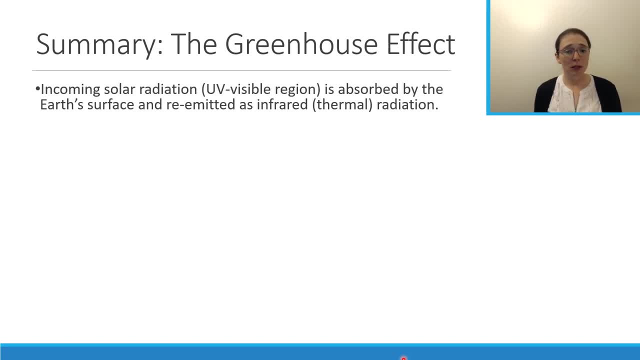 but just to recap briefly what we talked about, Incoming solar radiation from the sun is absorbed by the Earth's surface and it's re-emitted as infrared or thermal radiation. Greenhouse gases absorb some of this iron radiation and re-emitted, preventing it from basically escaping into space.